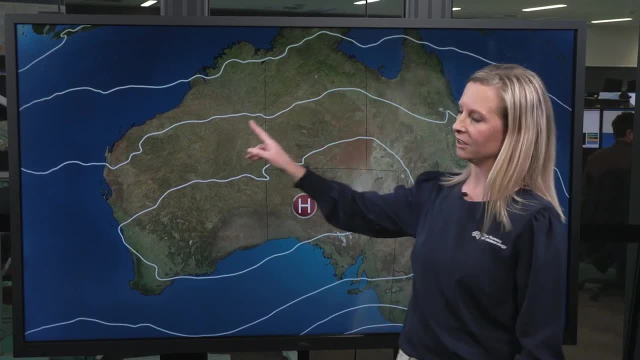 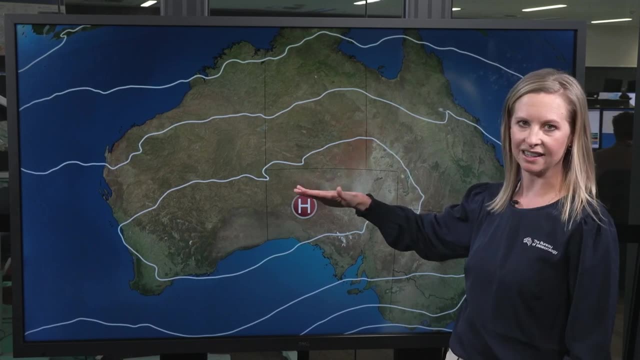 to drop And in the Southern Hemisphere the wind flows anti-clockwise around a high pressure system, And an interesting point is that the air in the centre of a high pressure system is sinking and that tends to lead to more settled weather conditions- Lows on the other. 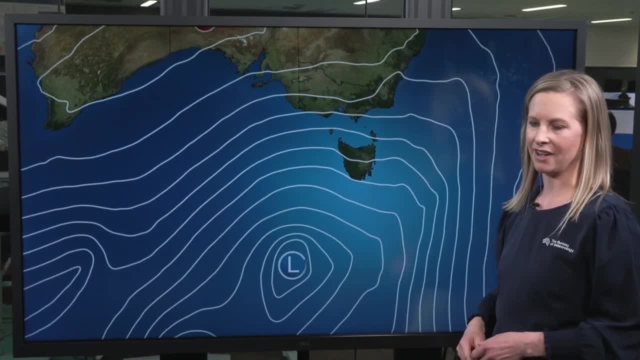 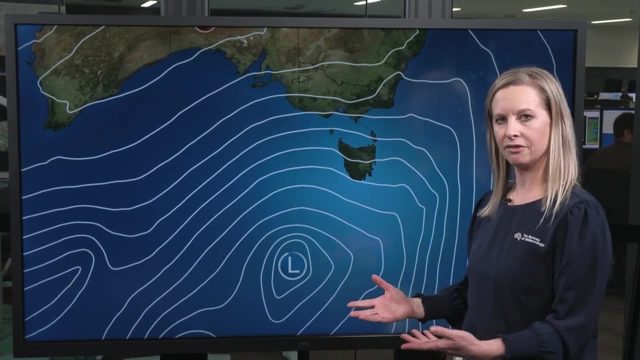 hand are like the bottom of a valley. They're the local minimums of atmospheric pressure, And in the southern hemisphere the wind flows clockwise around a low pressure system and in the centre of the low the air is rising. So lows on the map are normally associated with clouds, wet and stormy weather. 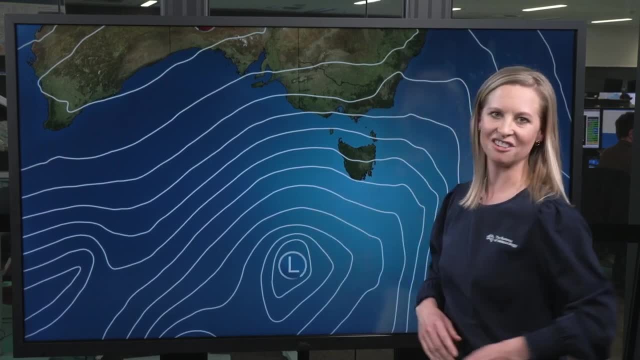 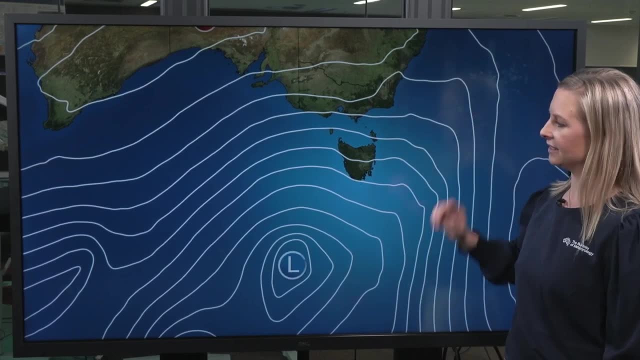 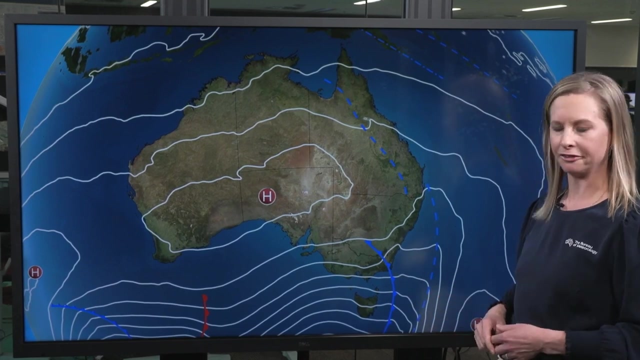 And you can also see that the isobars are quite close together around a low, so this is also indicating an area of windy conditions. Now it's time to talk about fronts. Now, fronts are the lines and shapes that you see on the weather map, and they indicate a boundary between two different air masses. 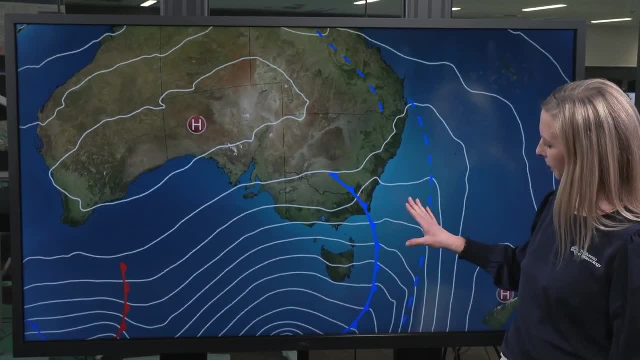 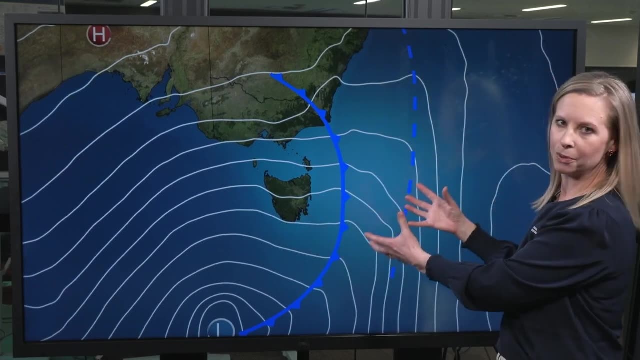 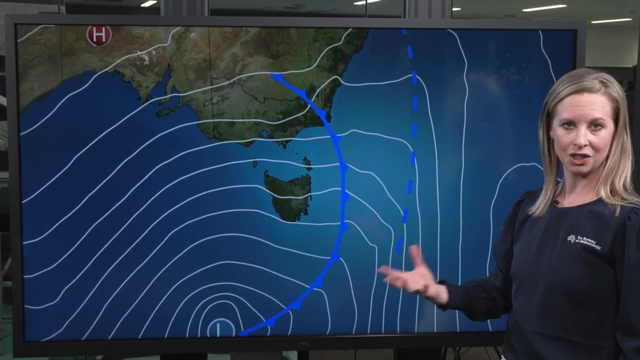 So we'll start by looking at the cold front, the blue line with the triangles. Now these indicate an area of where cold air is moving in and pushing warm air upwards. So we tend to expect to see a blanket of cloud along the leading edge of a front which can produce fairly consistent rain. 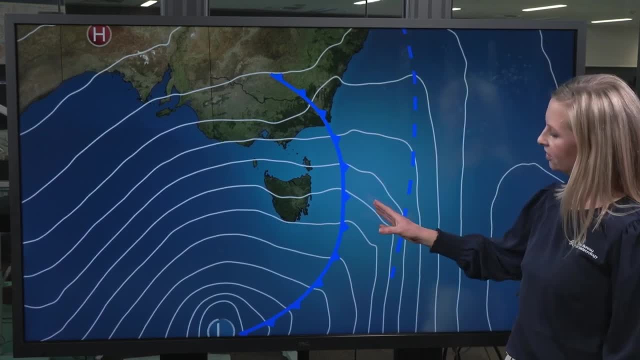 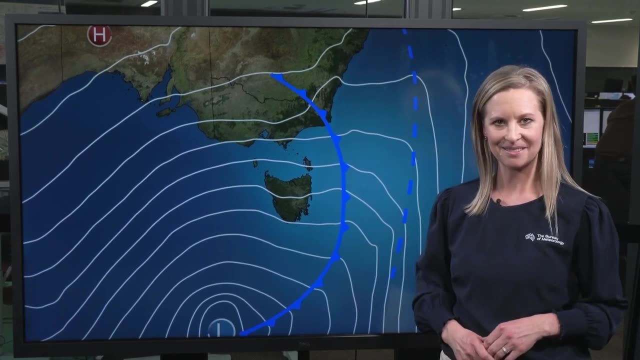 And as a front passes over you, you'll notice a change in wind direction and also temperature, And in summer there can be quite a sharp drop in temperature behind a cold front. Now the red lines and semicircles over here are indicating a warm front. 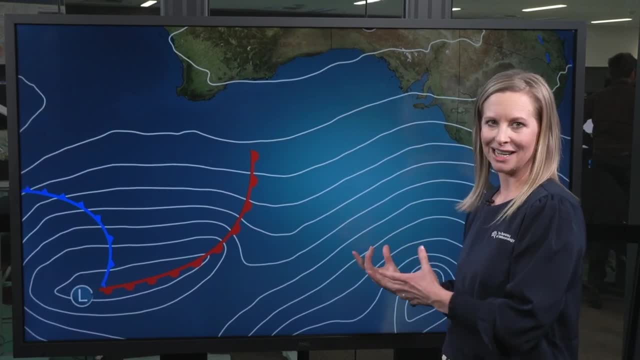 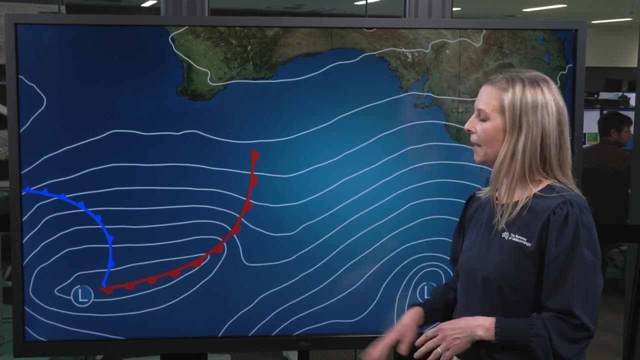 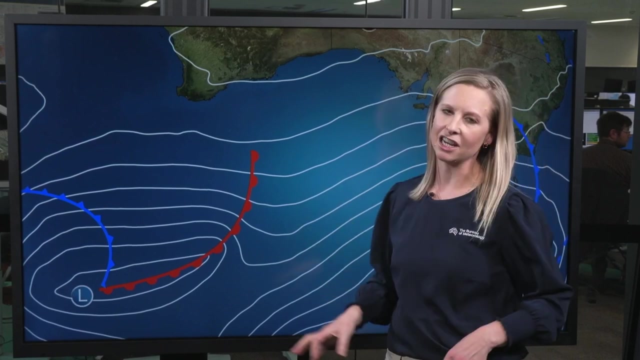 Now, a warm front is where warmer air will replace cooler air And, just like a cold front, there can be quite a marked temperature change when a warm front moves through, but typically less dramatic than what we would see with a cold front, And we do see these less frequently around Australia than we do cold fronts. 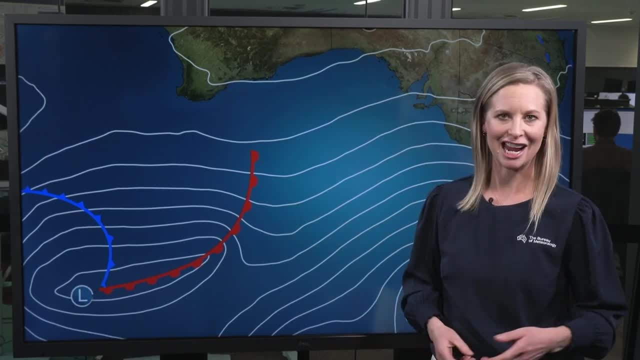 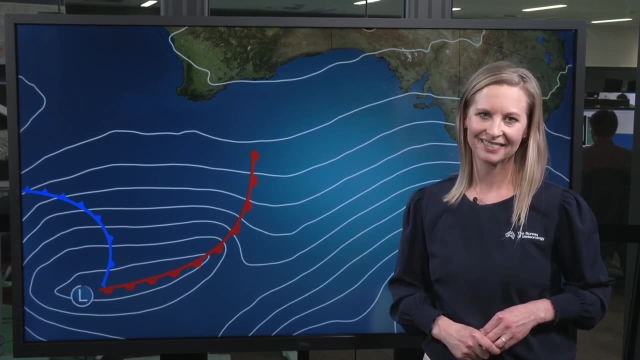 Now there's other types of fronts, too- stationary and occluded fronts, And if you'd like to know more about these, check out the blog linked. in our video description, We also see dashed lines like this one over here. Now this is an area called a trough. 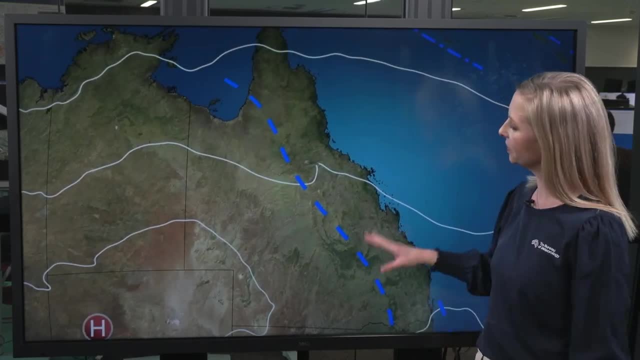 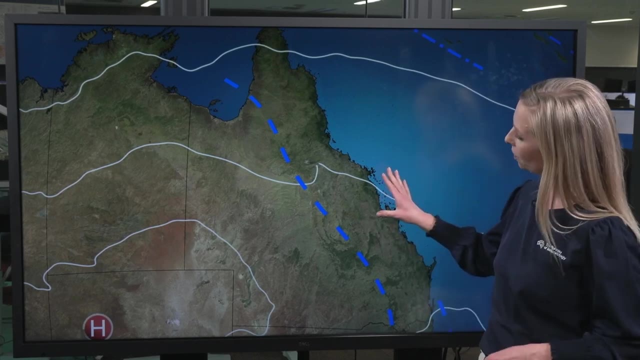 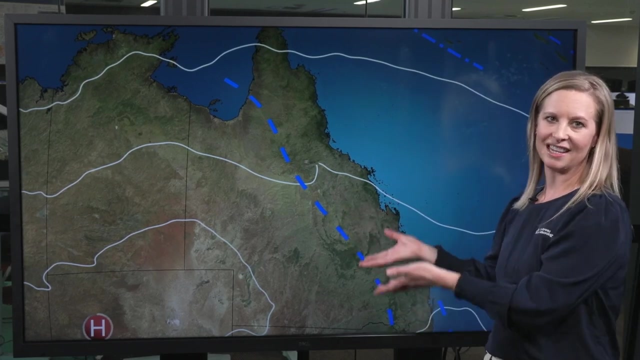 It's an area of relatively low atmospheric pressure compared to its immediate surroundings And, like cold fronts, troughs are separating two different layers. They're separating two different air masses- usually moist air on one side and drier air on the other- And as the trough moves towards the moist air, it causes the air to lift. 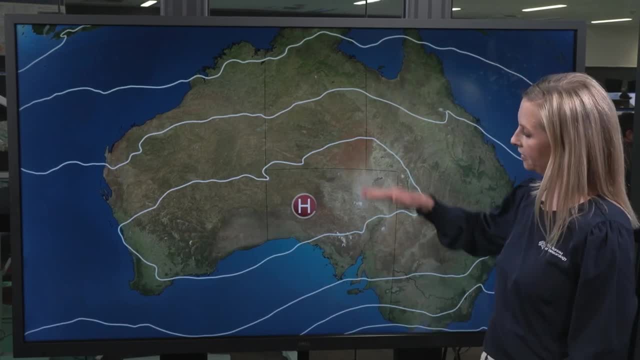 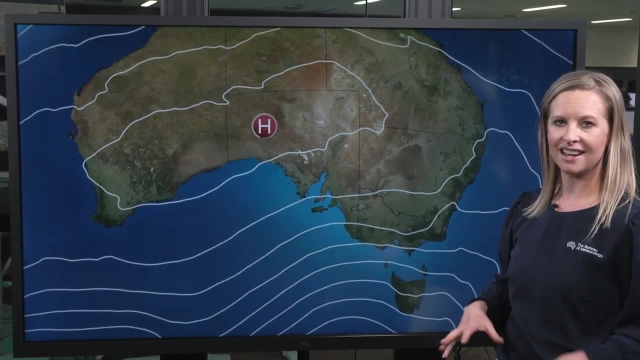 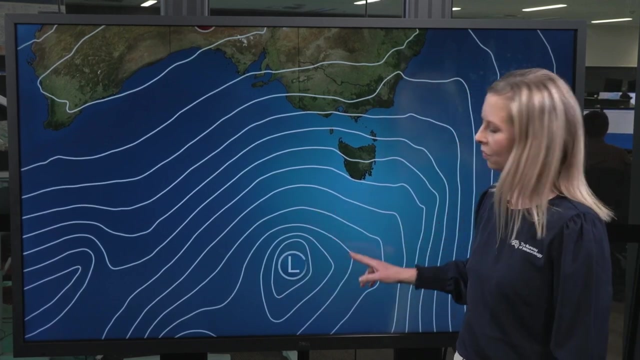 An interesting point is that the air in the centre of a high pressure system is sinking and that tends to lead to more settled weather conditions. Lows, on the other hand, are like the bottom of a valley. They're the local minimums of atmospheric pressure. In the southern hemisphere, the wind flows clockwise around a low. 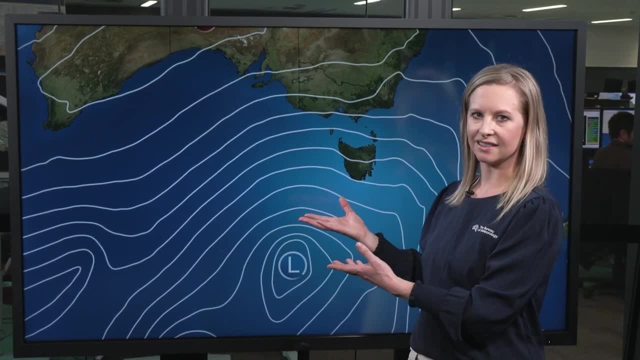 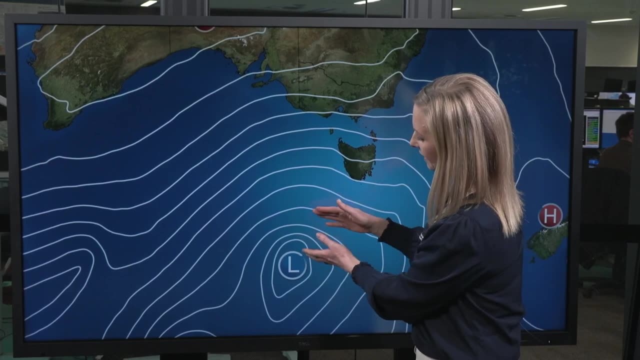 pressure system, and in the centre of the low, the air is rising. Lows on the map are normally associated with clouds, wet and stormy weather. You can also see that the isobars are quite close together around a low, so this is also indicating an area of windy conditions. 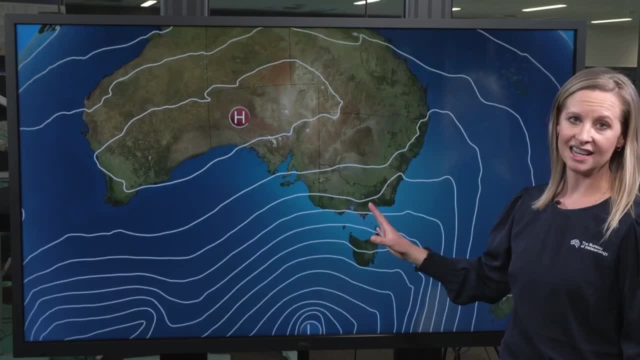 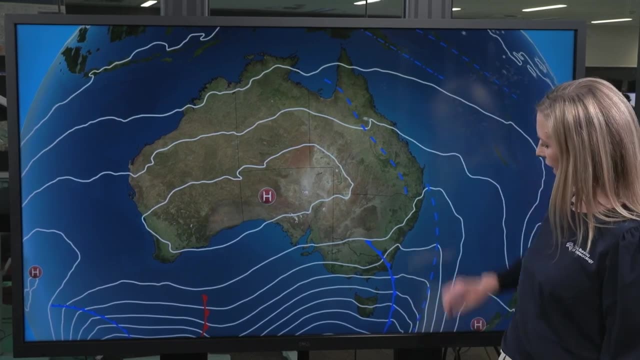 Now it's time to talk about fronts. Fronts are the lines and shapes that you see on the weather map and they indicate a bit of weather conditions. Fronts have a boundary between two different air masses. We'll start by looking at the cold front, the blue line with the triangles. 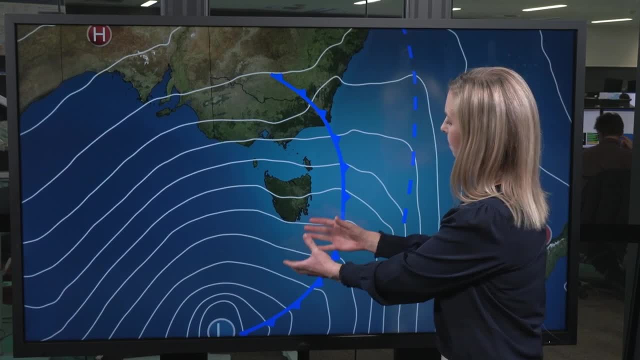 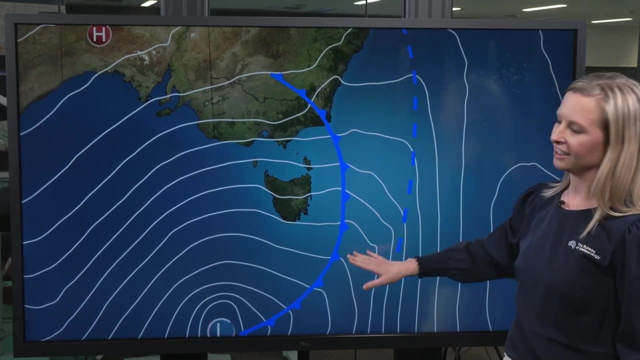 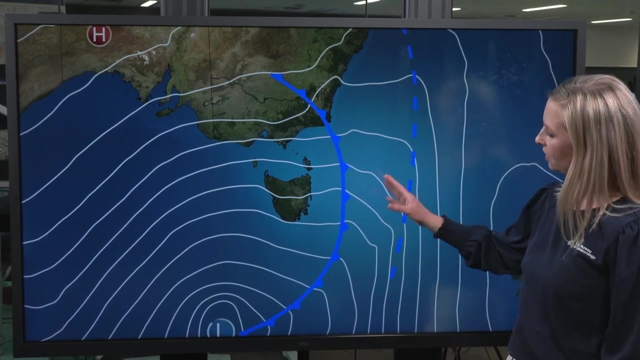 These indicate an area of where cold air is moving in and pushing warm air upwards. We tend to expect to see a blanket of cloud along the leading edge of a front, which can produce fairly consistent rain. As a front passes over you, you'll notice a change in wind direction and also temperature. 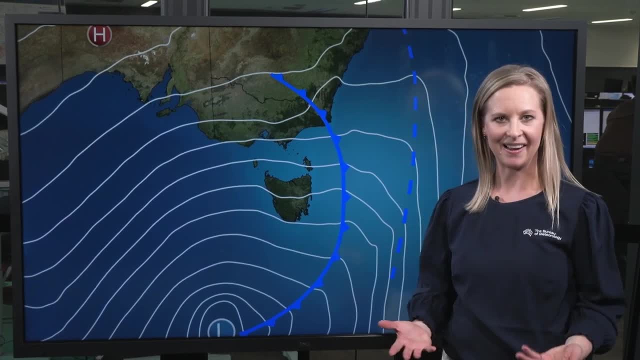 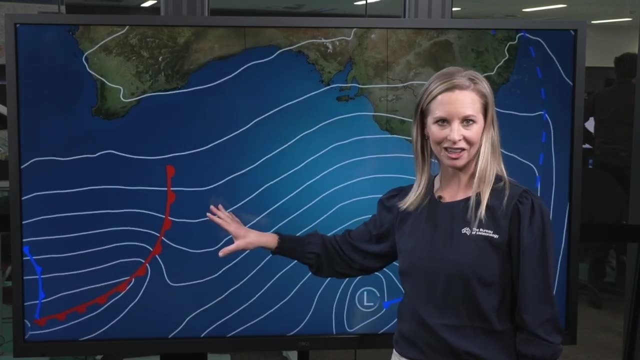 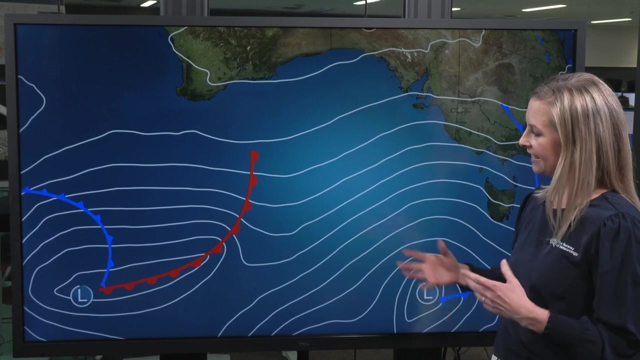 In summer there can be quite a sharp drop in temperature behind a cold front. Now the red lines and semicircles over here are indicating a warm front. Now a warm front is where warmer air will replace cooler air And, just like a cold front, there can be quite a marked temperature change. when a 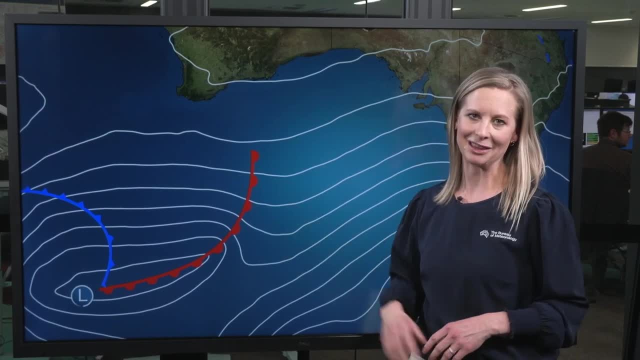 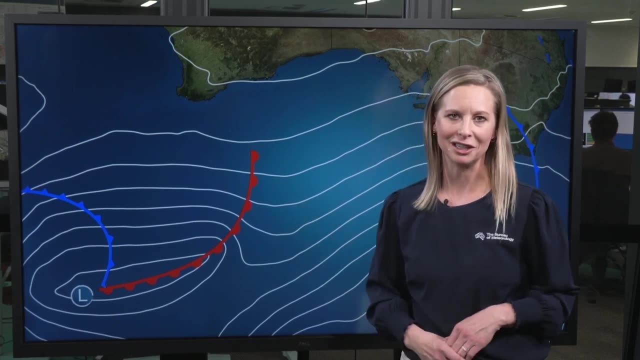 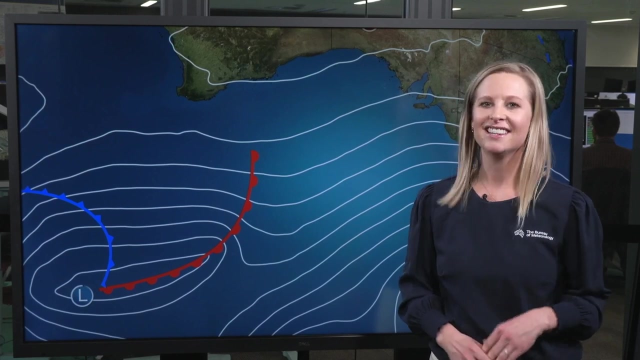 warm front moves through, but typically less dramatic than what we would see with a cold front, And we do see these less frequently around Australia than we do cold fronts. Now, there's other types of fronts too- stationary and occluded fronts, And if you'd like to know more about these, check out the blog linked in our video description. 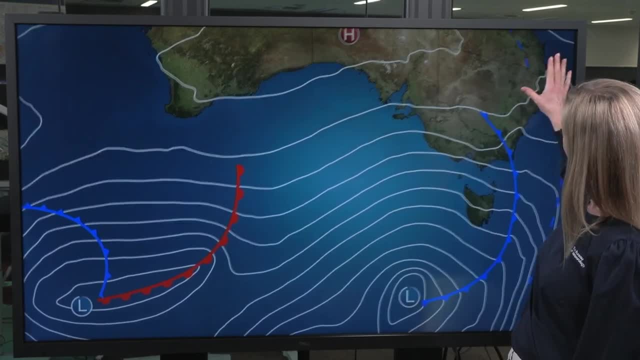 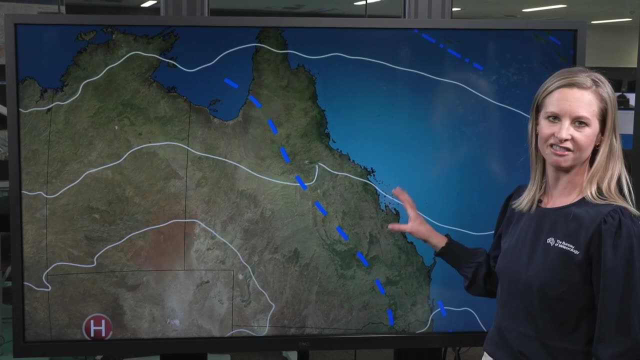 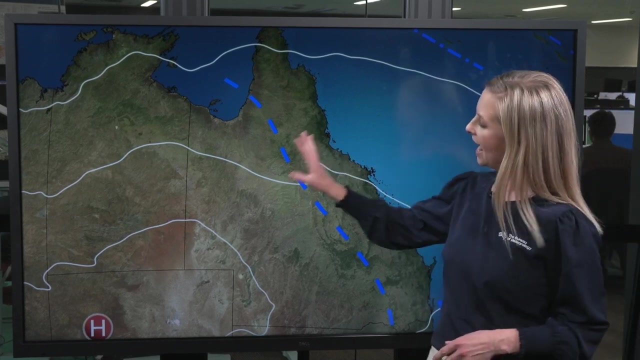 We also see dashed lines like this one over here. Now this is an area called a trough. It's an area of relatively low atmospheric pressure compared to its immediate surroundings And, like cold fronts, troughs are separating two different air masses: usually moist air on one side and drier air on the other. 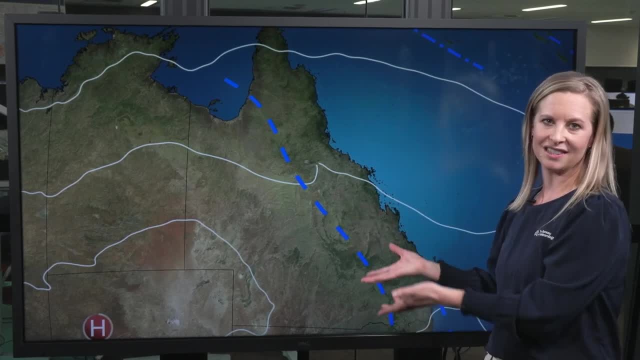 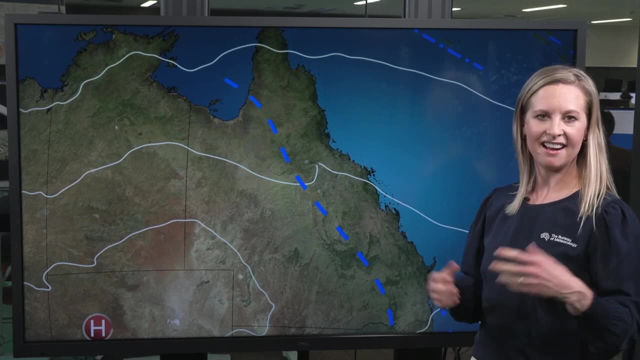 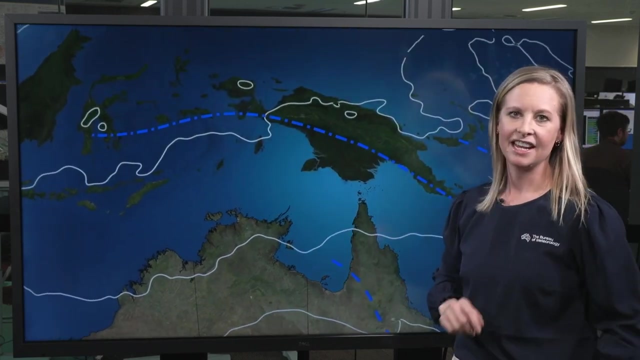 As the trough moves towards the moist air, it causes the air to lift, And so we see cloud and showers and thunderstorms, often developing on a trough. Now, another type of trough that we see in the Australian region is the monsoon trough, shown by this dot dashed line.